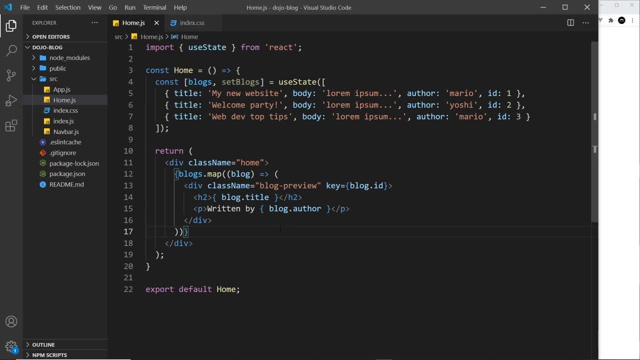 we'll do that in the form of props. so, for example, on the home page we might be able to do that in list all of the blogs and show a preview for all of the blogs starting with the latest one. but on a search page or a search component we might only show the blogs that match the search term. so the 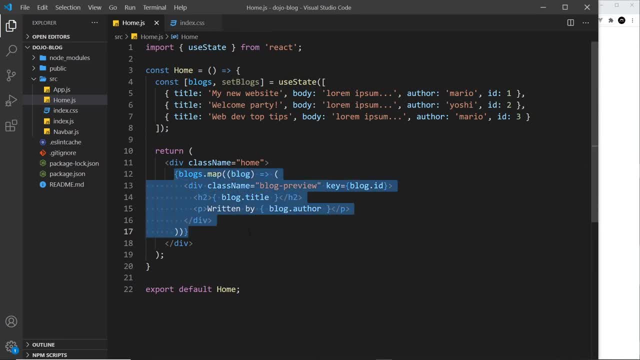 data is going to be different, the structure is the same, but the blogs that we use are going to be different. so we can pass in data into these external components as well, in the form of props- and we'll see those shortly- but first of all, let's create an external component called blog. 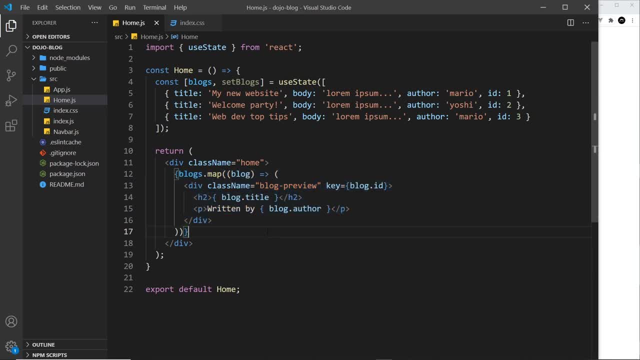 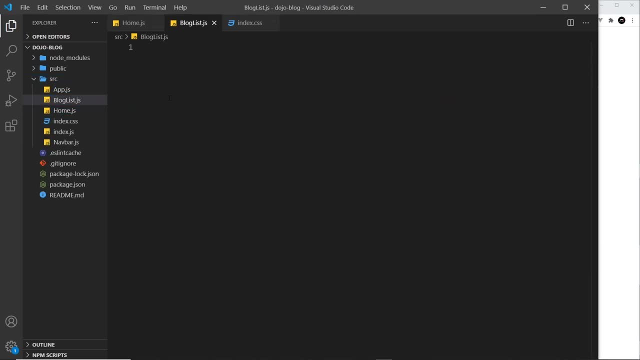 list to house all of this logic or all of this template. so then, let's start by creating a new file called blog listjs, and then inside here we need a stateless, functional component. hit tab and we'll call this blog list, like so. all right, so the template is just going to be the template. 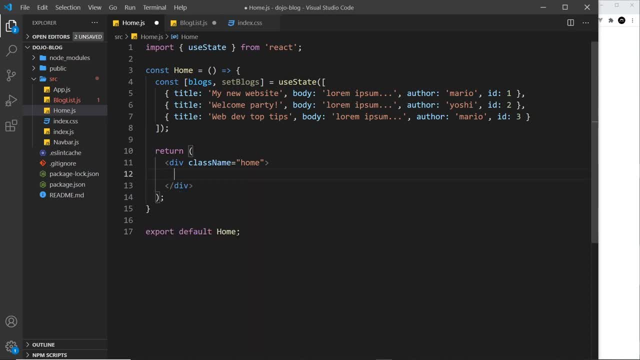 that we have currently right here, so let's grab it from here. i'm going to cut it and then down here. i'm going to first of all create a div with a class of blog hyphen list, like so, and i'll place it inside here, like so. so we're still cycling through the blogs. 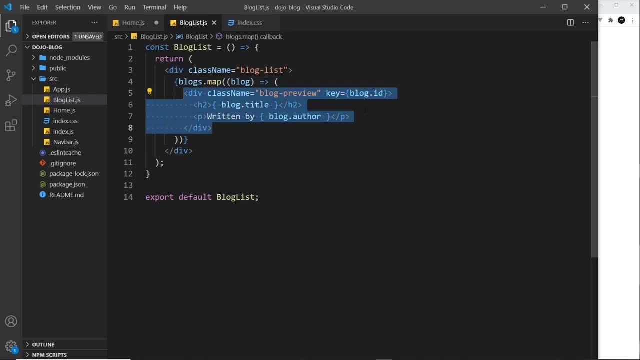 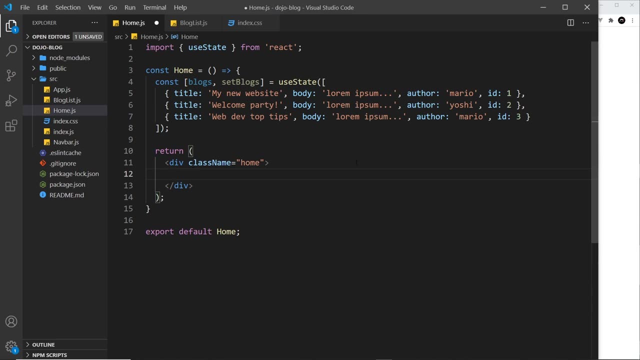 and we're still outputting a bit of template for each one. so let me save this. and now we want to nest this blog list component inside the home component right here. so i'm going to say blog list and notice i can click on this and it. 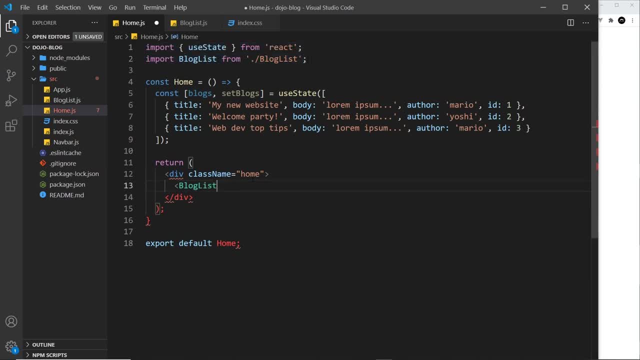 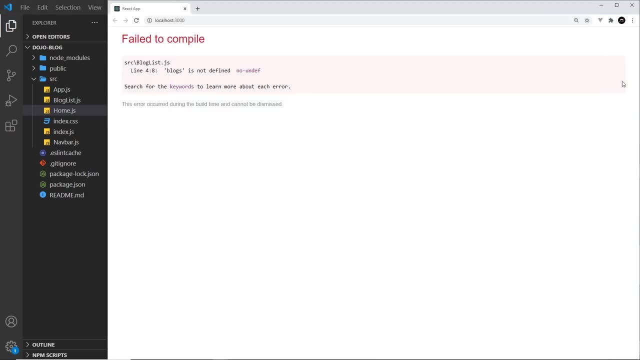 is going to auto import it for me at the top. so let me close this off now and there is a problem with this and we'll see that in a second. but let me save it and try and preview it and we get an error and it says blogs is not defined. so that's because in the blog list, 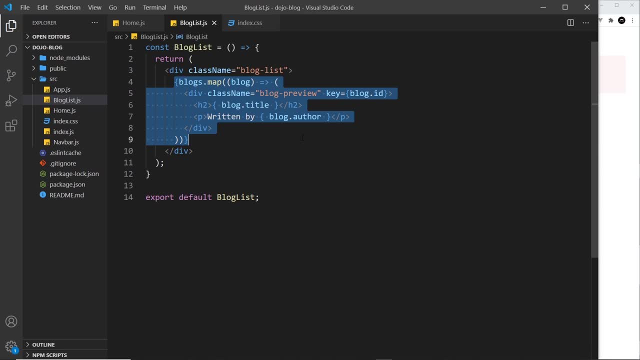 component. we're trying to map through the blog. so we're using data here, but it doesn't know what blogs is, because the blogs data is not defined in this component. we can't just use any data in here where, for instance, let's say, this is my website, i'm going to write blog, i'm going to 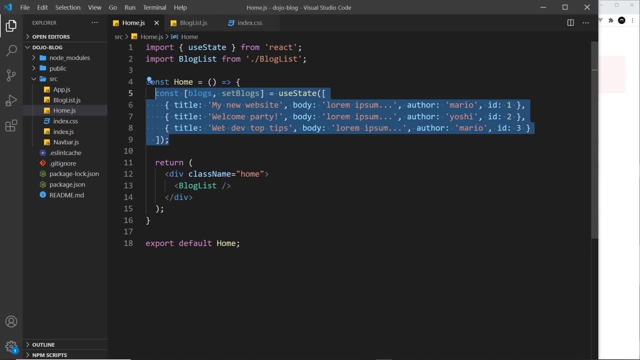 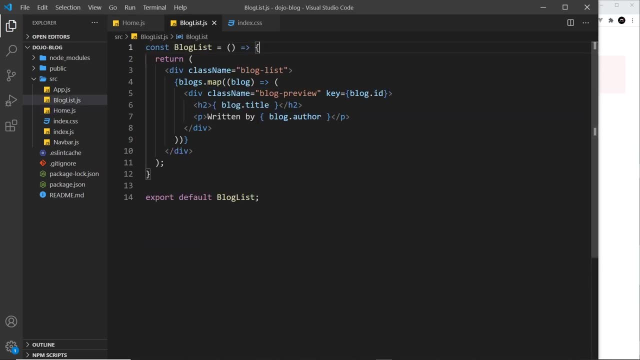 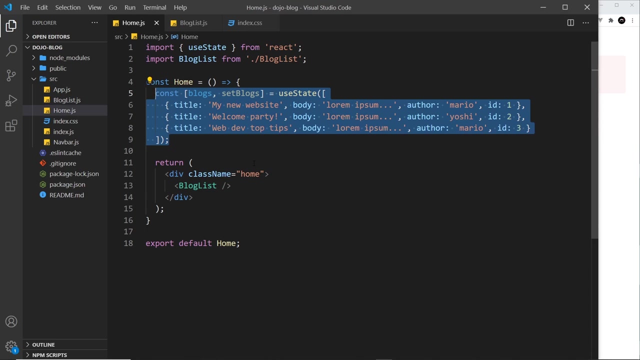 plug in this blog list component where it's defined right here, because it can't reach that okay. so there's a couple of different ways around this. the first option is to redeclare all of this data inside this component instead of home. so we delete it from here and we place it over here instead. the 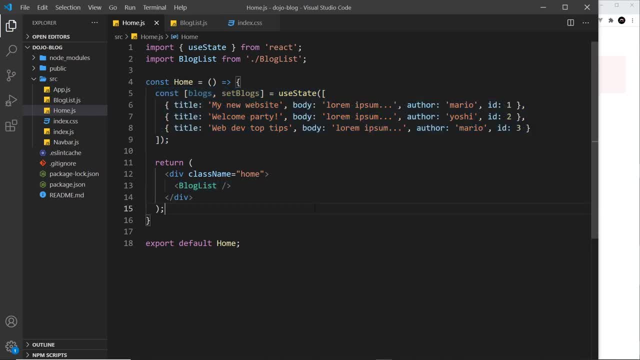 second option is to use props, whereby we pass this data from this home component into the blog list option. props for three reasons. first of all, it's going to make our blog list component more reusable, and we'll see exactly how later on. second, it allows me to still use this data in the home. 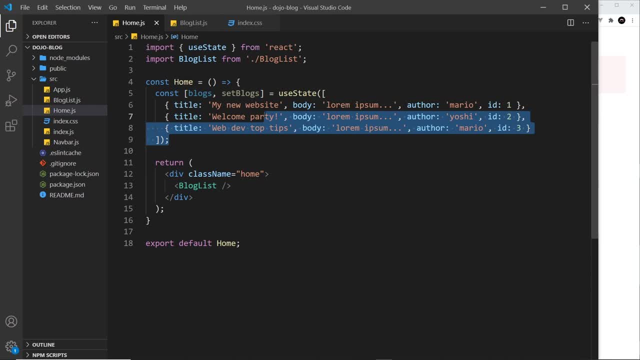 component later on, if I need it in the future, because the data is still going to be declared here. and third, it allows me to show you how to use props. all right, so props are a way to pass data from one component, a parent component, into a child component. so this is the parent component. 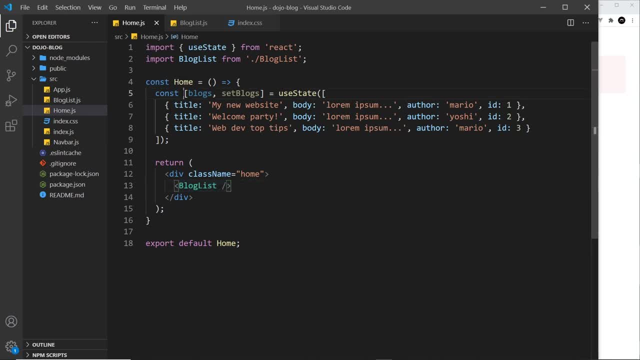 and this is the Child component right here. so we want to pass the blogs data into. the blogs is by making a property name on this tag, so you can call it what you want. I'm going to call it blocks, since that's what we'll pass in and this is going to be a dynamic value. so 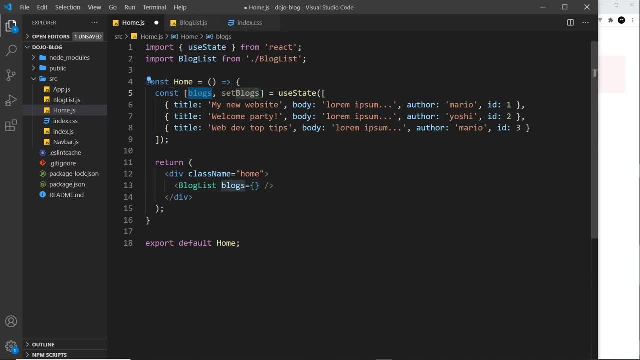 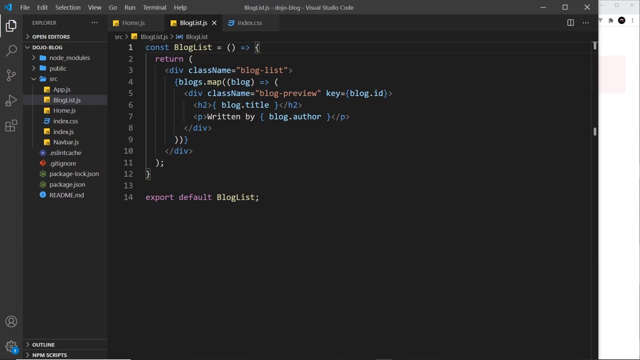 curly braces and the value is going to be blocks like so. so just pass that in. and now this is being passed into the blog list component as a prop. this right here is a prop, so we need to receive it inside the blog list components and we get access to an. 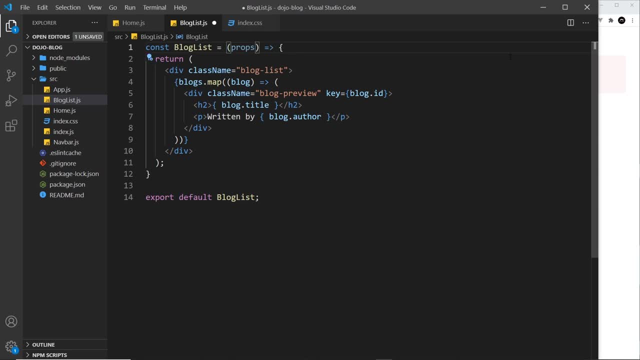 argument inside this function, inside the component called props. so now this property, right here, blogs is going to be on this props object so i could access the blogs from it. so let me do this. i could say: const blogs is equal to propsblogs, like so, and what i'm going to do is just log. 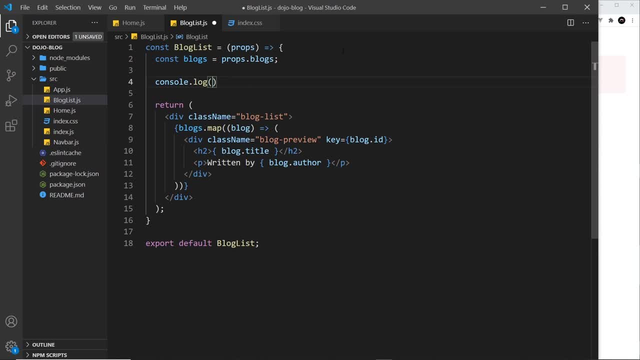 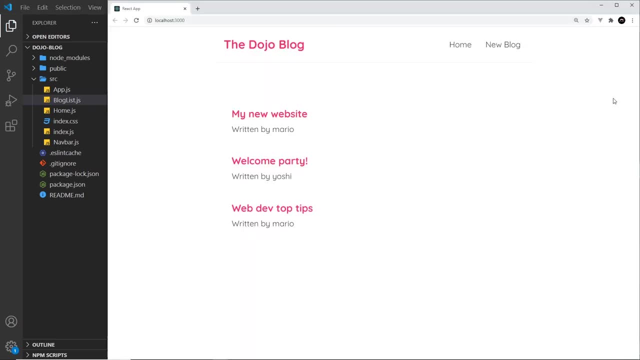 that to the console. so i'll say consolelog and in fact we'll log out the props as a whole as well and blogs, all right, so let's come over here and inspect this. notice first of all, if i wrong me here, is that i have a response that says props, prop is not being accessed. so i'm going to. 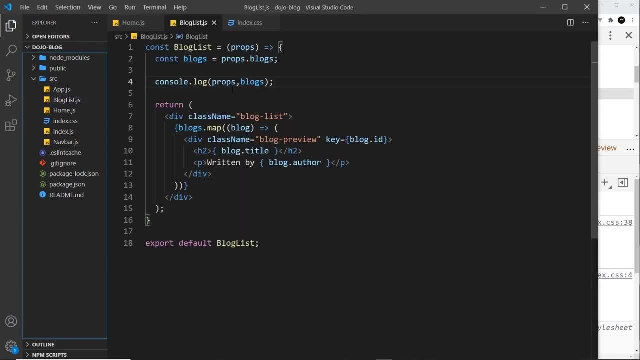 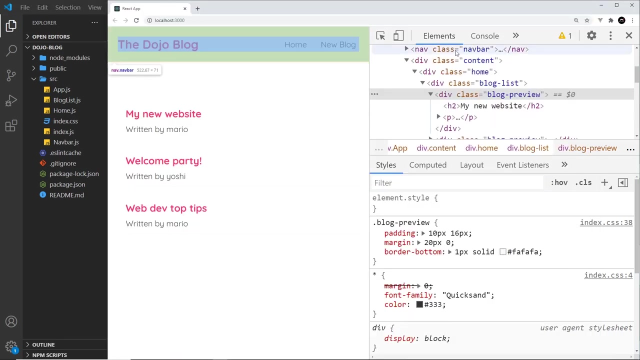 refresh. everything's still working because we're now passing the blogs into this component and we're grabbing the blogs right here, storing them in this constant and then we're cycling through that constant at the bottom. so this works now as it should, but let's go over here and see what's. 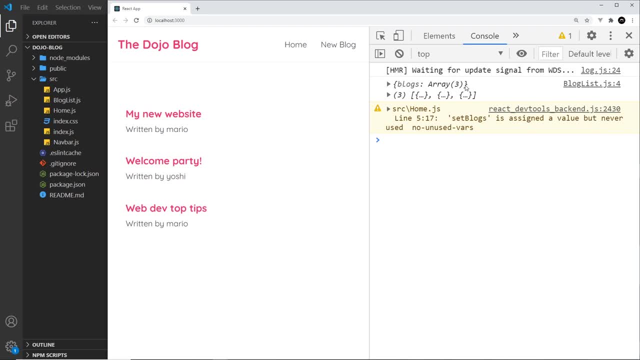 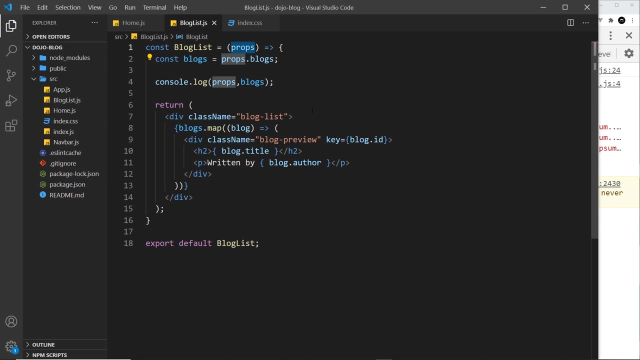 in the console. so this top one, right here, this is the props object and you can see it has a blogs property only, which is an array, and down here this is the blogs themselves. all right, so any props that we send through into a component are attached to this object, which we automatically get. 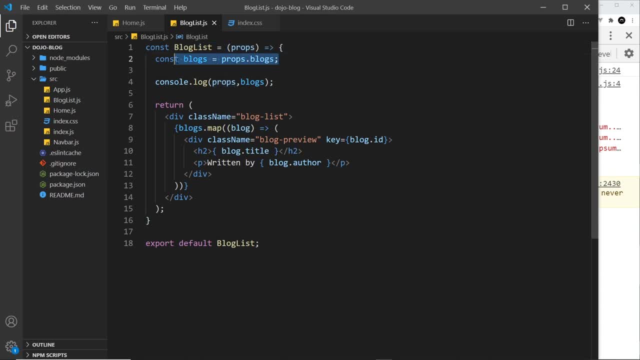 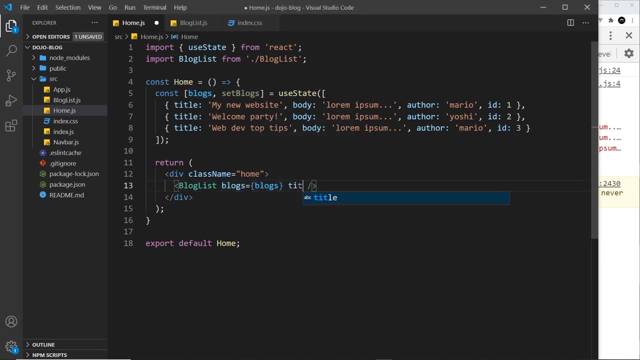 as an argument in the component and we can access them. now we can pass multiple props if we want to. so i could pass in another prop, for example, called title, like so, and set that equal to some kind of string. now it can be a dynamic value which is stored in some kind of variable. 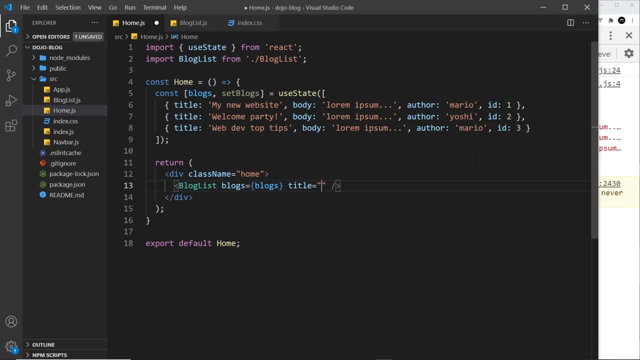 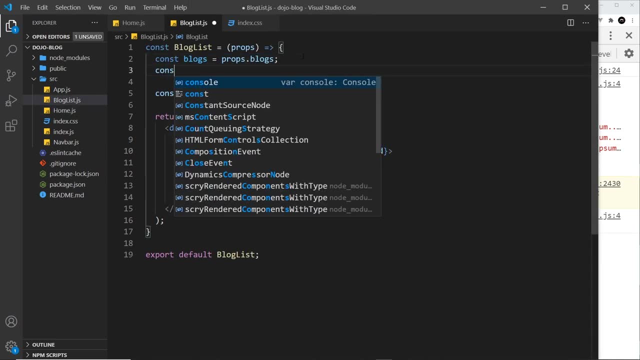 but i'm just going to pass in a string value, so the title is going to be all blogs, and then what i could do is access that as well from the props. i could say: const title is equal to props dot title. all right, so let me delete this consolelog. we don't need that anymore. now, what i'd like to do 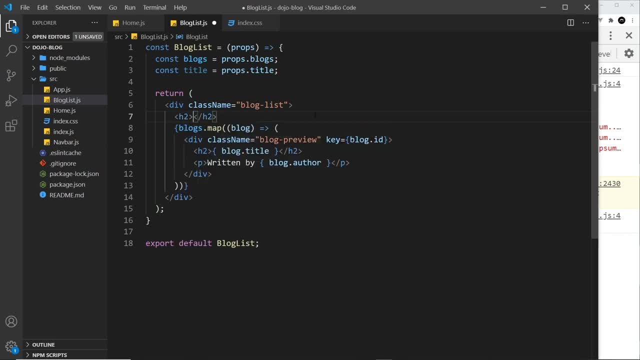 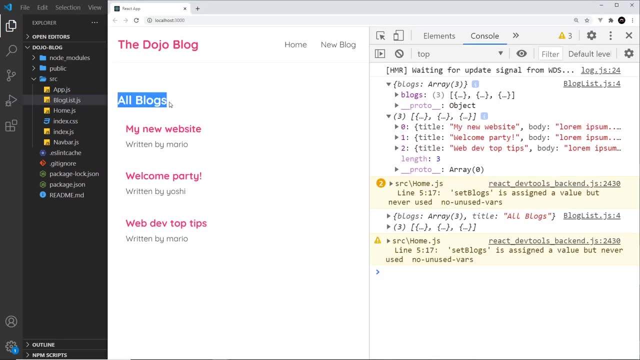 is output this title above the blogs. so i'll do an h2 and then inside there we'll do the title. so if i save this now and preview, we can see we get the title as well. and if we change that, just add an exclamation mark, then it's going to. 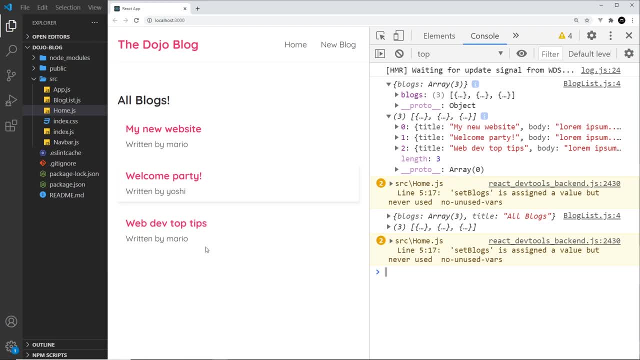 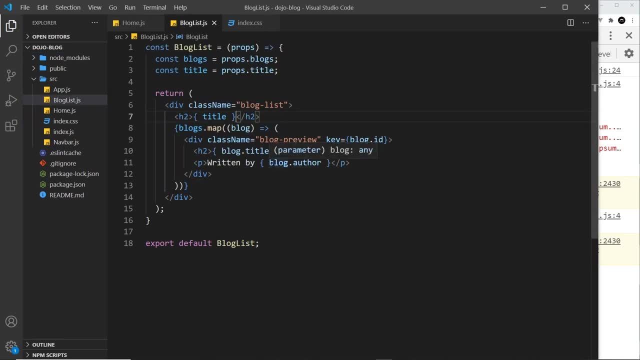 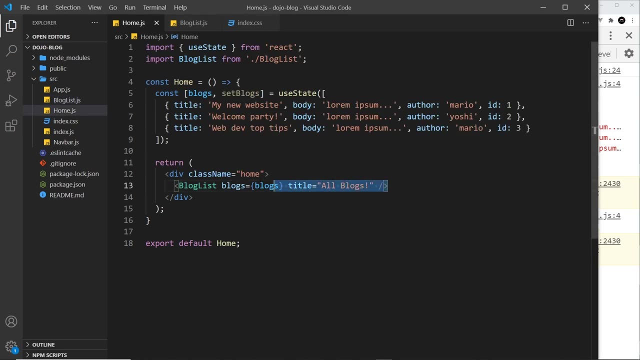 update. so then that's how we can make a component to take in props data and then use that data inside that component. now i said before, it makes this component, now this blog list component, more reusable, and it does. we can now use this blog list component anywhere in our application. 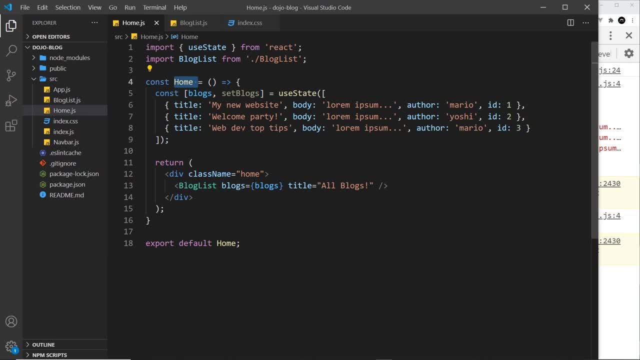 whether that's in the home components or in a different page component later on, and i'm going to demonstrate that in the next tutorial. but before we finish this video, i want to show you one more thing. if we go to the blog list right here, we can see what. 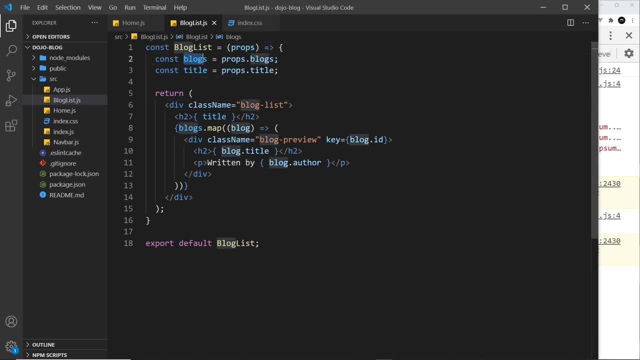 i accept, in this props object and then we're grabbing the different properties from that props object right here and storing them in these variables. now, an easier way to do this is to destructure the props directly inside these parentheses, so i could comment these things out and i could get rid of this and i could.